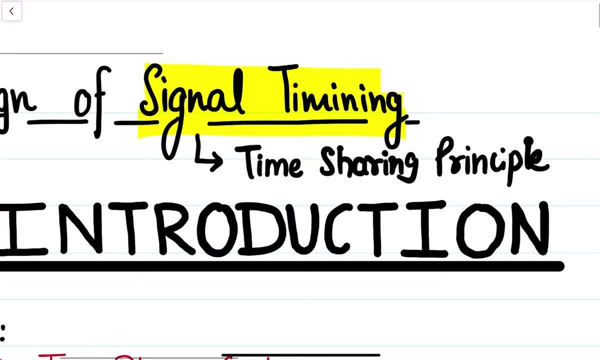 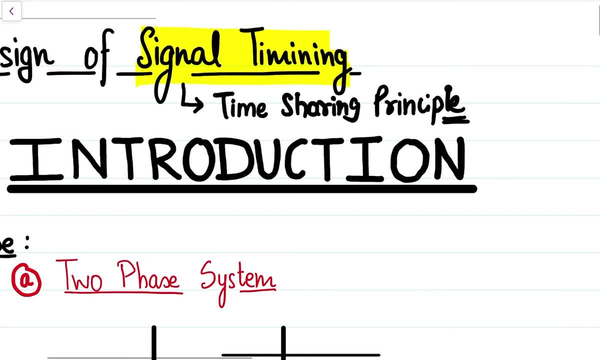 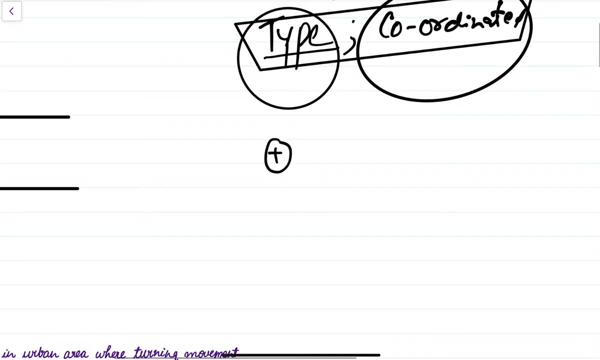 That in a road section, all the vehicles should get optimum amount of time to cross the intersection Right. So if we talk about the positive parameters related to traffic signal time or the installation of traffic signals, the positive aspect is that it separates the conflict movement of vehicles. 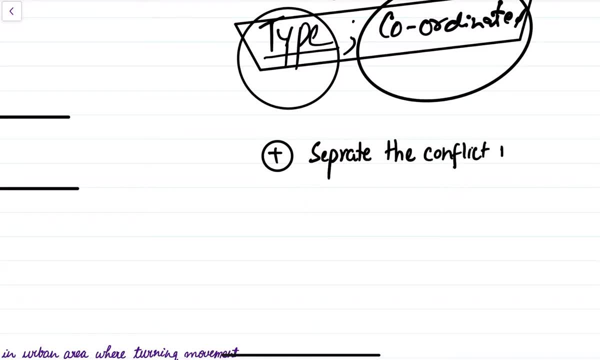 It separates the conflict movement of vehicles. So we have discussed about the conflict points in an uncontrolled intersection And by installing the traffic signals we try to separate the amount of conflict that can be created with respect to the uncontrolled intersection, where the traffic is allowed to move in whatever way they want. 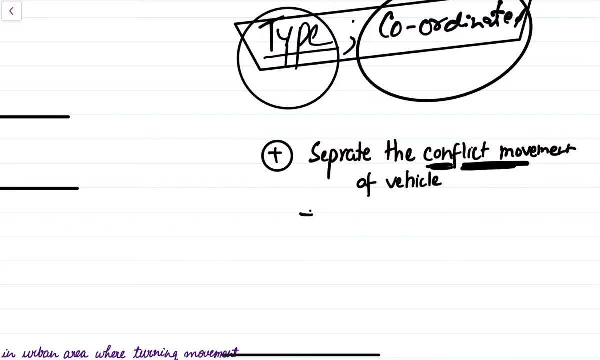 By doing so, another positive aspect is created, That is, it increases. it increases the road capacity. It increases the road capacity Right The limitation. the limitation that is attached to the traffic signal is that if the traffic signal time is not decided in a in a given way, 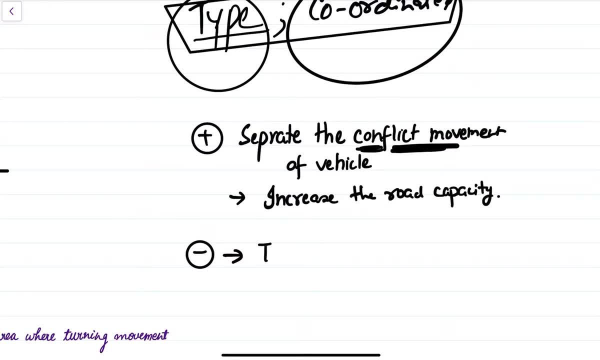 Then it will lead to too much delay time. It will lead to too much delay time. Alright. This is the limitation that is attached towards the traffic signal timing design. Alright. So this is the positive and this is the negative, Alright. 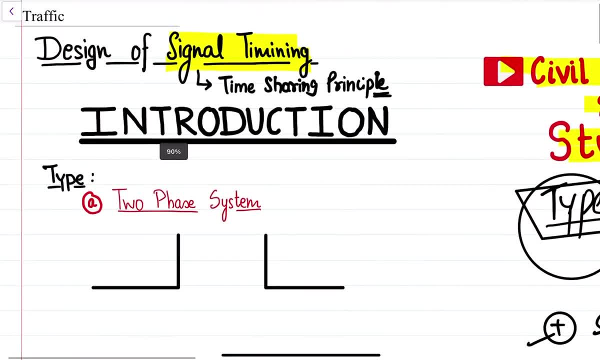 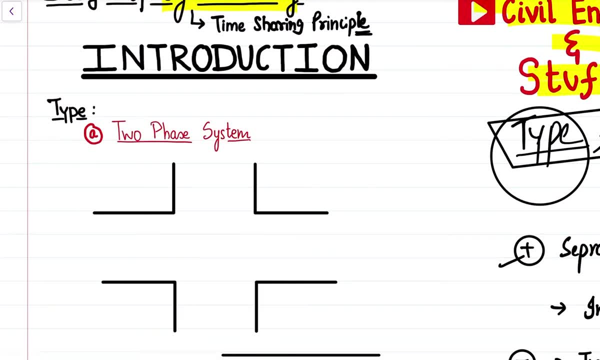 So let us start with the basics about the design of traffic signal timing. So, talking about the traffic signal timing, The traffic signal is designed in such a way that it can either work in a two-phase system or it can work in a four-phase system. 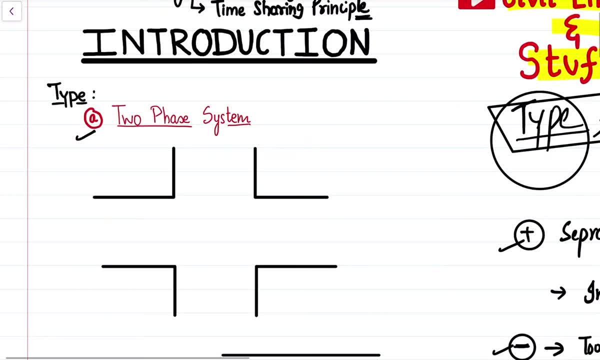 So in a two-phase system the movement of traffic is such a way that either in an intersection, the traffic at a time can move in one road like this. This is the first phase In a. in an intersection, the traffic at a time it can either move like this: 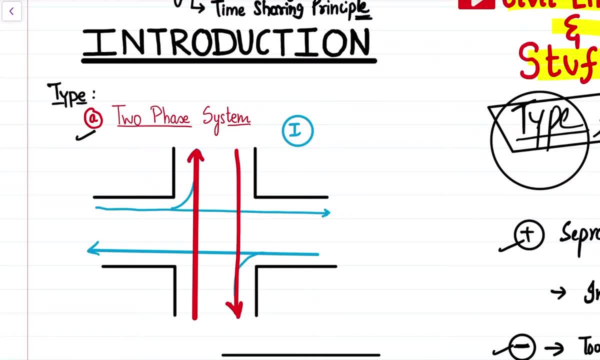 This is the first phase, And in a second phase the traffic can move. the traffic can move like this: Alright, This is the second phase of movement that can be done in an intersection by installing the traffic signal. So when this happens, this is called as the two-phase. 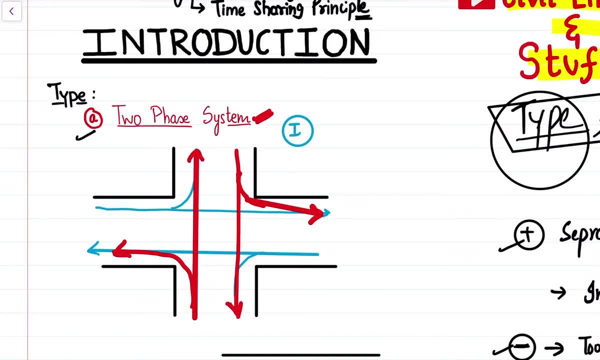 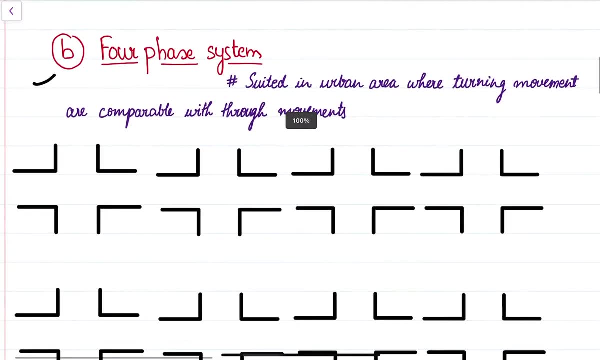 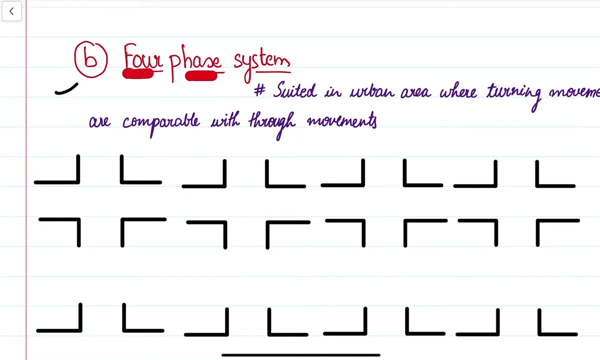 system. Through this, by designing these two-phases, the traffic can be allowed to move. But in case where the traffic volume is very high, so see the two-phase, four-phase traffic signal system is decided. So in a four-phase traffic system, these type of traffic phase systems. 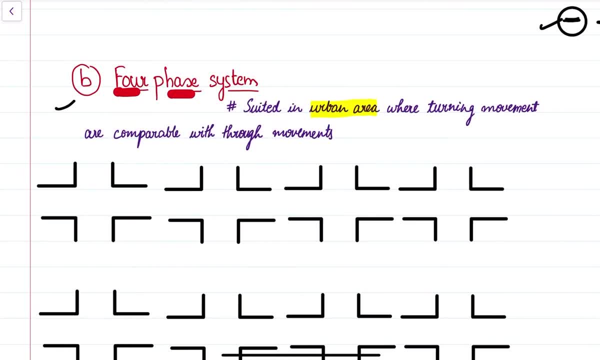 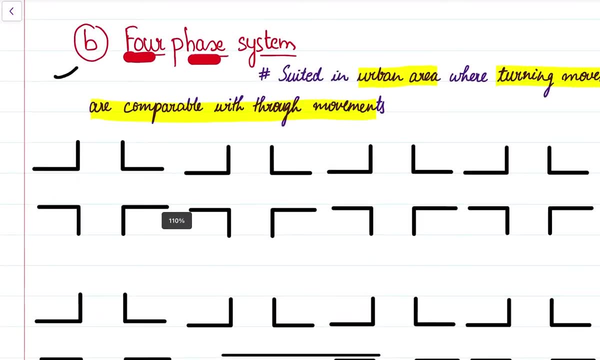 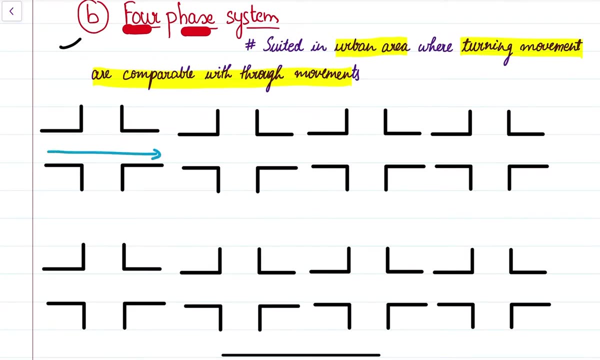 are used in urban areas where the traffic volume is very high and the turning movement is comparable with the throw movement. So in a four-phase traffic signal movement, what happens is in the first phase the traffic can go like this. It is like this: 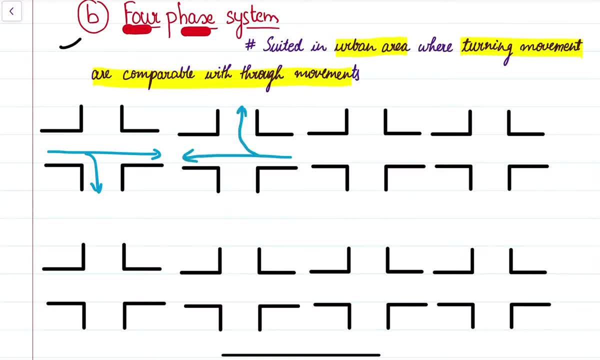 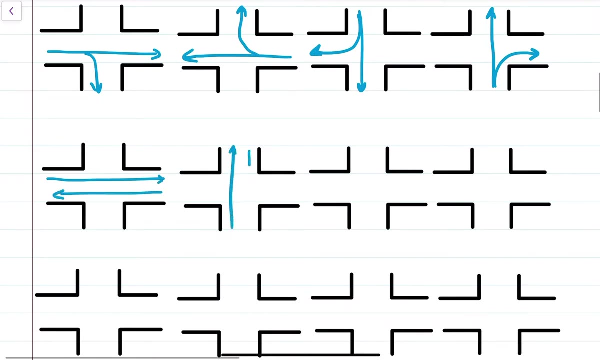 It can go like this, It can go like this And it can go like this. Right, The another way, or another possible way in which the traffic can move is traffic can move like this In the first. this is the second way the traffic can move. 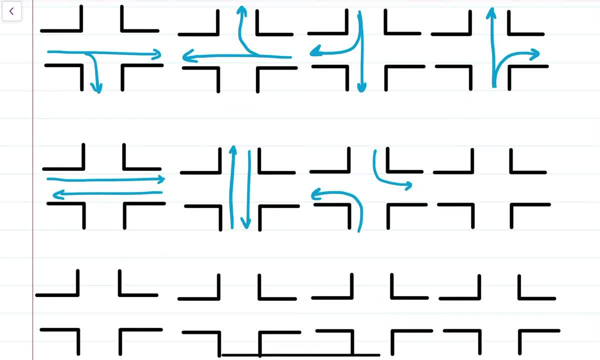 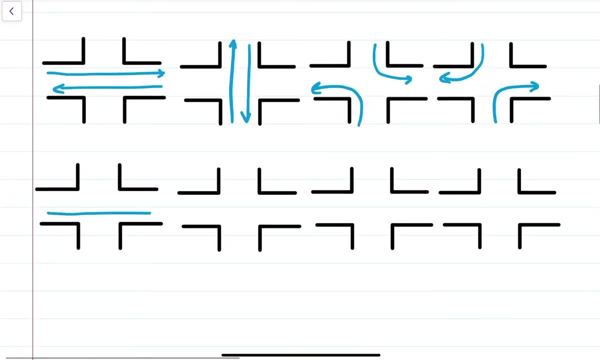 The third way the traffic can move And this is the fourth way the traffic can move. This is another possibility, the second possible way of providing a four-phase traffic signal system. The third possibility can be it can move like this: The traffic can, at a time, can move like this: 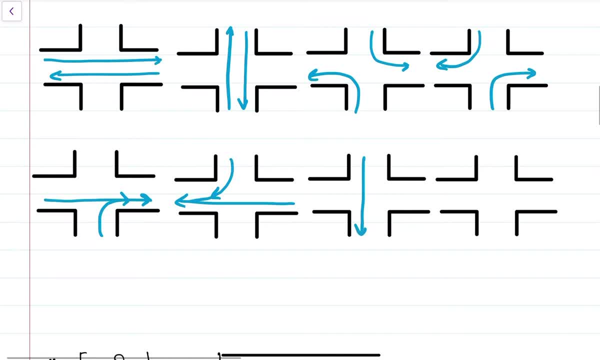 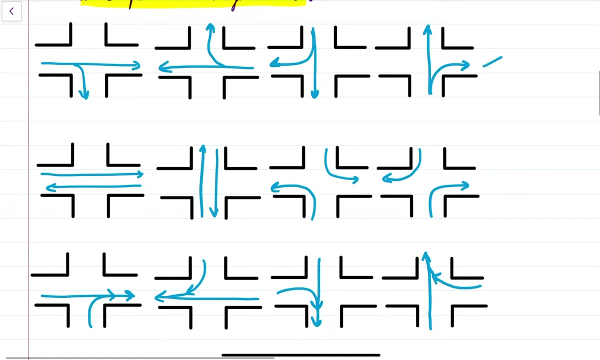 The traffic can move like this. And the fourth phase: in fourth phase, the traffic can move like this: Alright, This is the third possible way where the four-phase traffic signal can move, Alright. So in a four-phase, these are. these are the three possible ways. 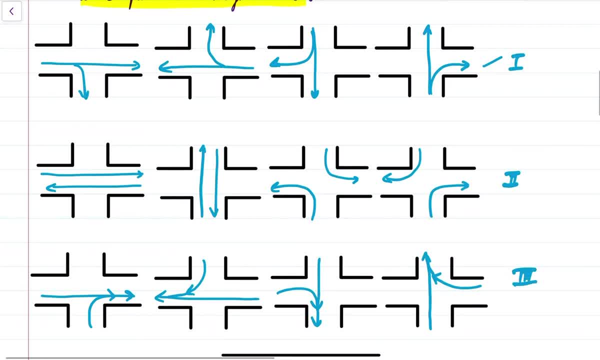 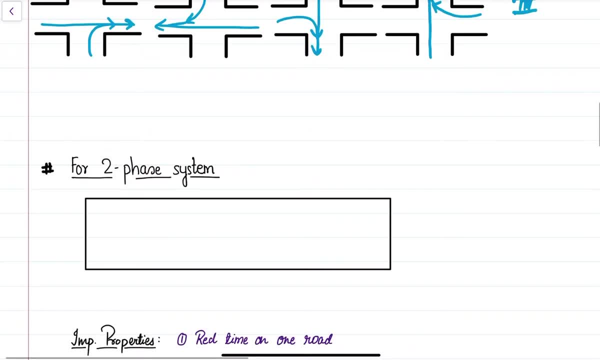 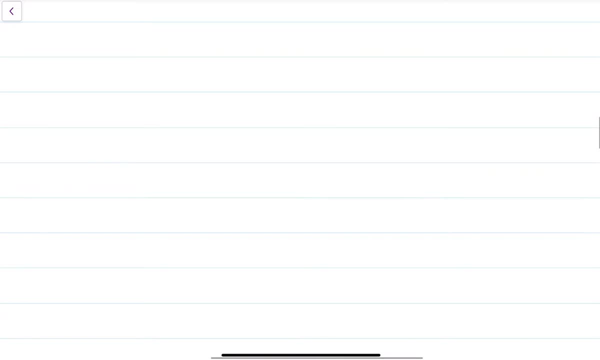 First, second and third way in which a four-phase traffic signal can be designed. Alright, So let us discuss about two-phase system first. Alright, Let us discuss about two-phase system first. So, in a two-phase system, let us say that this is our intersection, over which we have. 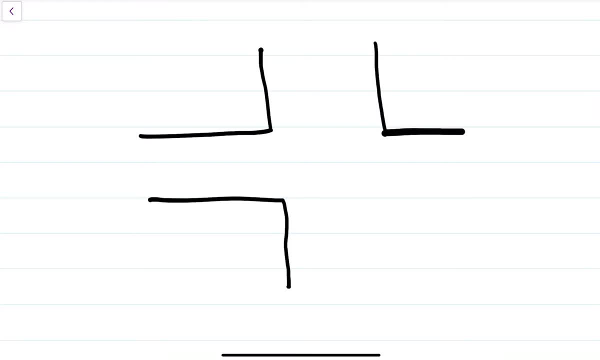 to install the traffic signal. This is an intersection, this is road A and this is road B, over which we have to install a traffic signal. Alright, So we know, in a traffic signal, we have three lights, Right, We have three lights. 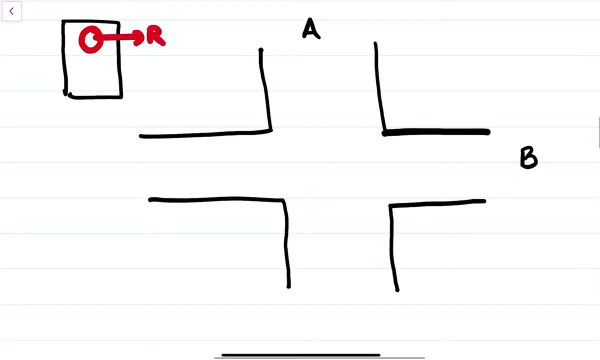 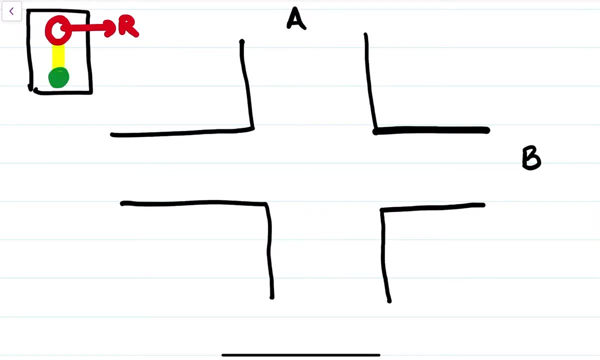 We have the red light, We have yellow that we can also call as the amber, And then we have the green light. We have red, We have yellow or what we are going to refer it as amber, Alright, And then we have green light. 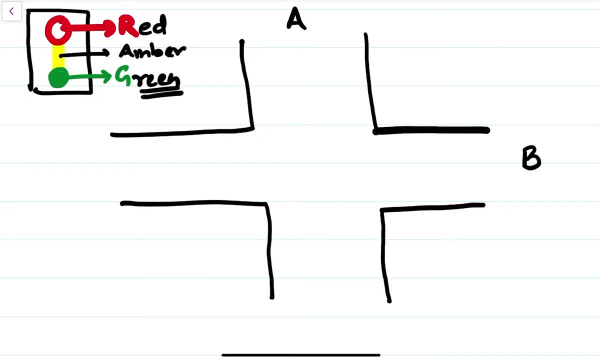 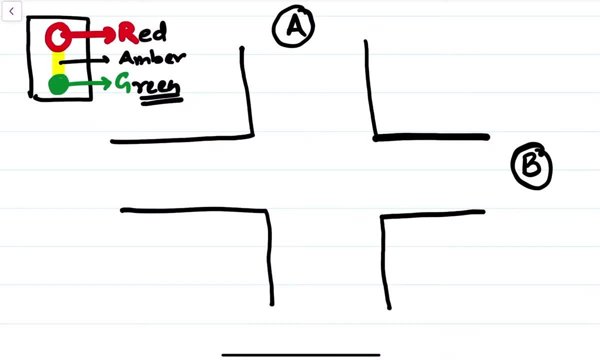 Alright. So now listen very carefully. We have road A, we have road B. Now let us say: in road A we have allowed the movement of traffic. In road A we have allowed the movement of traffic. This means that now in road A- this is, we have green light. 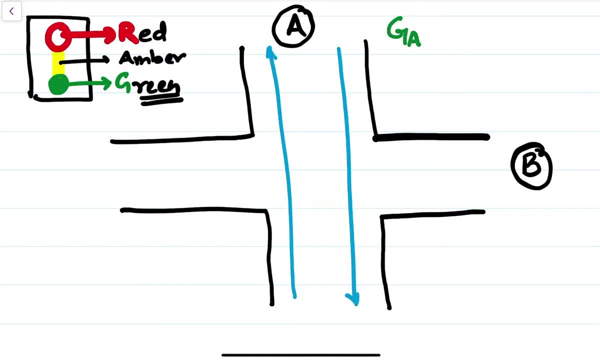 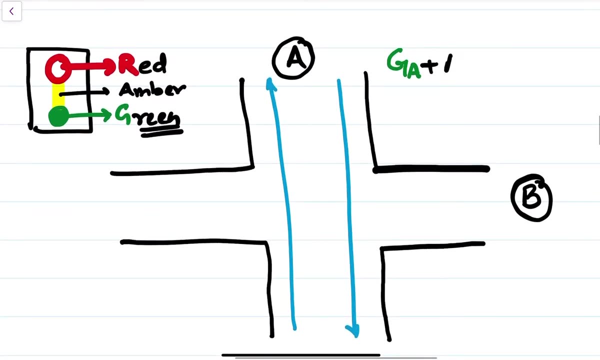 Right. We have green at road A Right. So when there is green at road A, after green, we will have, we will have amber, After green we will have amber. Amber is a traffic light that is used for warning. 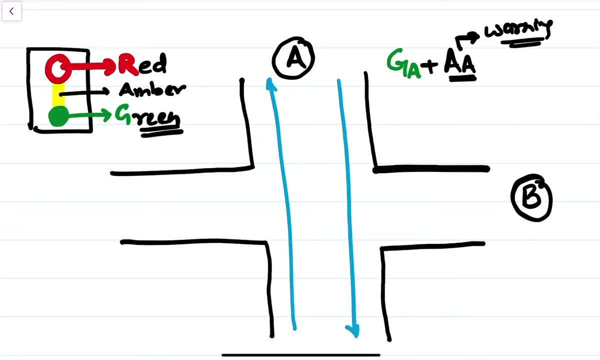 Right, It is used as a warning for the ongoing traffic. Actually, that is right now moving in road A to tell that now it is going to be red. So we will either cross this intersection or stop and wait for the next green light to come. 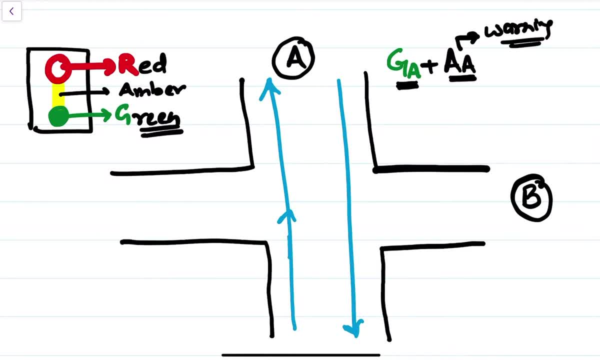 Right. So if you think, when it is green and amber at road A, so what do you think will be in road B? I will again repeat: if it is green and amber in road A, so in road B what will be the traffic light? 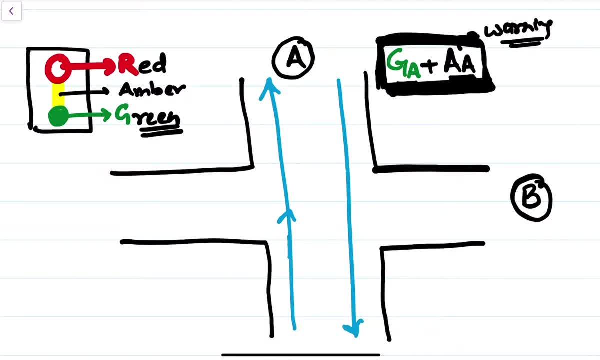 In road B the traffic light will be red. Right The traffic light at road A will be red. They will be red at road B- Clear, Because the traffic has to stop in road B in order to ensure that there is safe passage for road A. 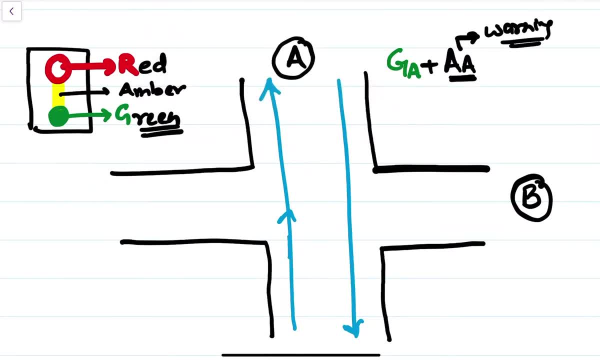 Likewise. Likewise When it is when we are now allowing the movement of traffic in road B, When we are allowing the movement of traffic in road B, So of course the traffic at road A has to stop. So they will be red at A in order to ensure that it is green at road B. 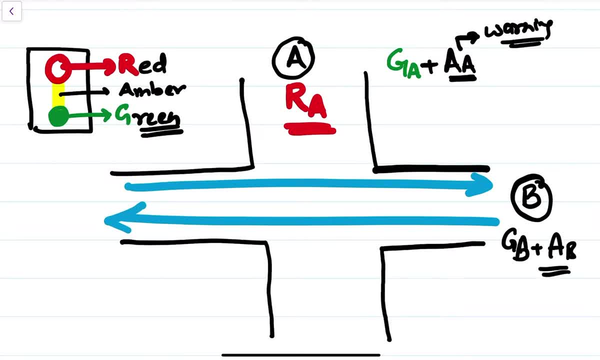 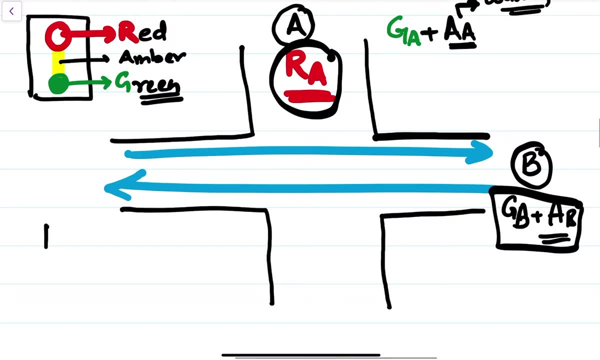 And followed by amber at road B, Right Green at road B and amber at road B, At that time they will be red in road A Clear. So if I say, if I say when it is red in road A, so at that time in road B, what kind of traffic light it will be? 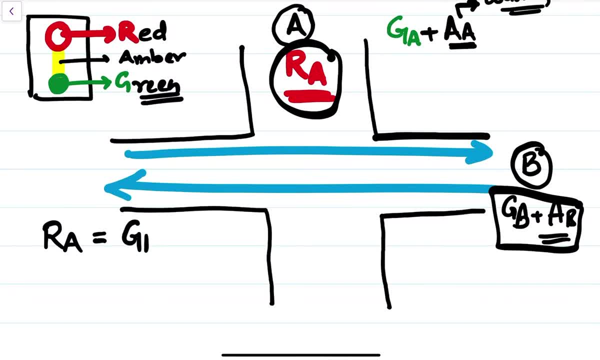 It will be green at B, Green at B, followed by amber at B. When it is red at road A, that is, the traffic is at stop, then only the traffic can move in road B. So red at road A is equal to green at road B, plus amber at road B. 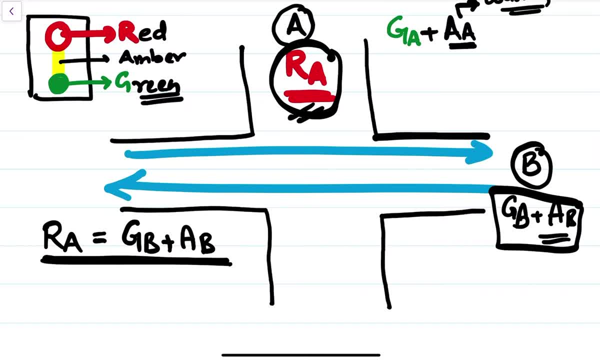 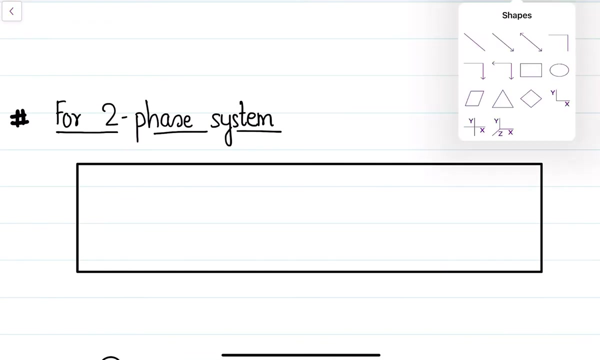 In the similar fashion. in the similar fashion. The red In the similar fashion, the red at road B. when it is red at road B, it will be green at road A as well as amber at road A, Right? So if we show this in a two-phase system, if we want to show this in a two-phase system, 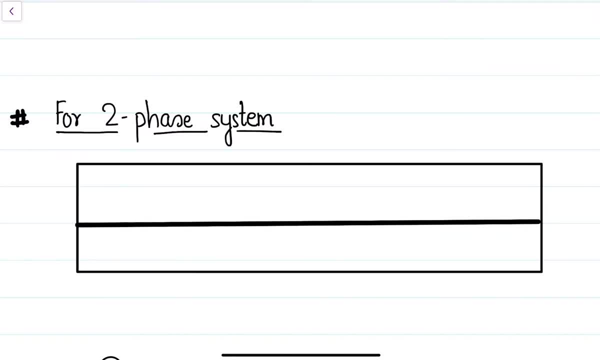 Let us say, let us say: this is, this is road A And this is road B. Right, This is road A and this is road B. So when it is, when it is, let us say: it is red. 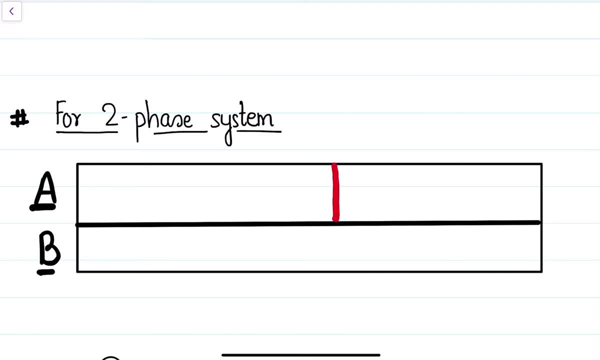 When we have, when we have, when we have red at road A, When we have red at road A, What will be in road B? In road B, we will have green in road B and we will have amber in road B. 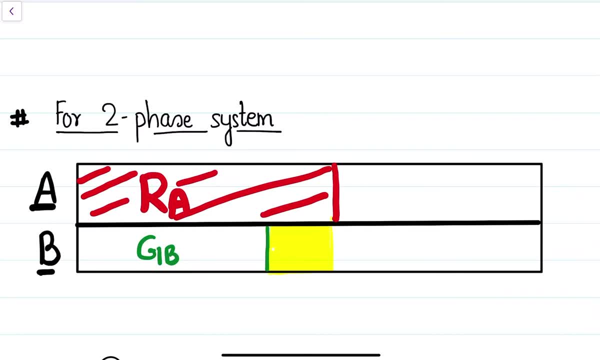 We will have green in road B as well as we will have amber at road B Right And at the same time, if we say we have red in road B, If we say that these are time periods where day is red at road B, then in road A we will have green in road A and we will have amber in road A. 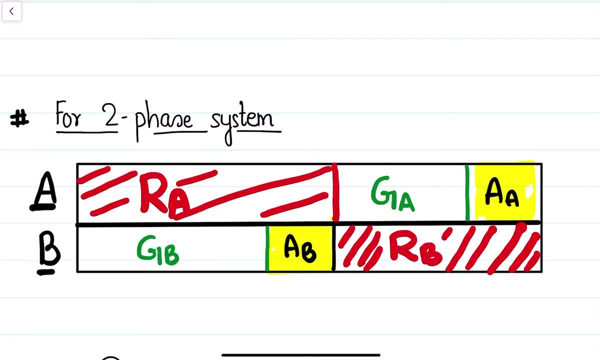 Clear We will have. we will have green in road A as well as we will have amber at road A, Right? So this is how a two-phase system is represented, in the form of kind of a bar chart. Okay, All right. 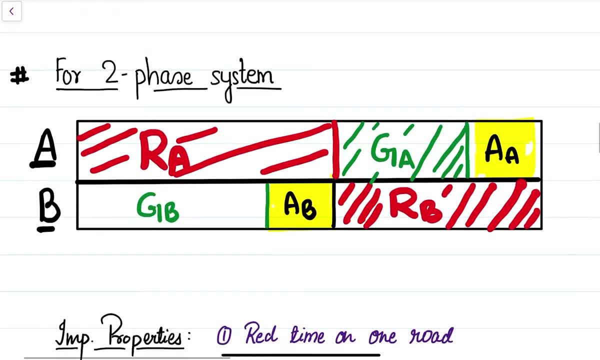 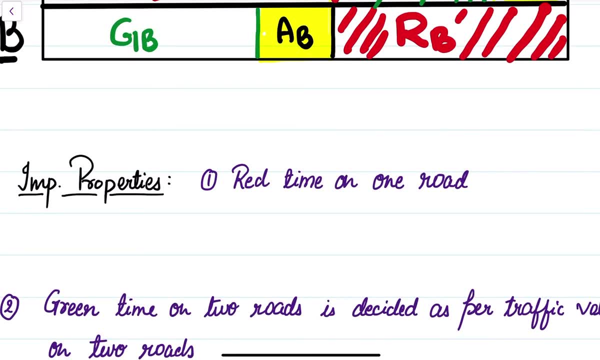 Now let us discuss a few more important points. So we have discussed about this: When it is red time in one road, When it is, let us say, red time in road A, So it will be- then red time is equal to what? 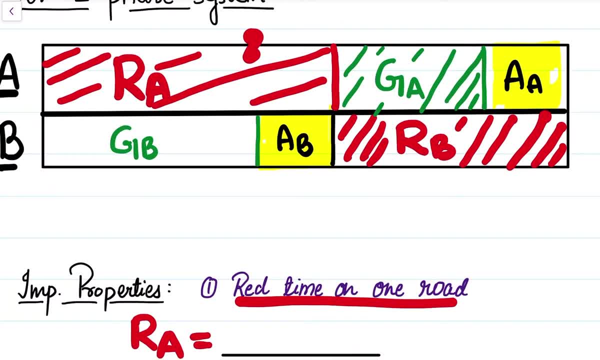 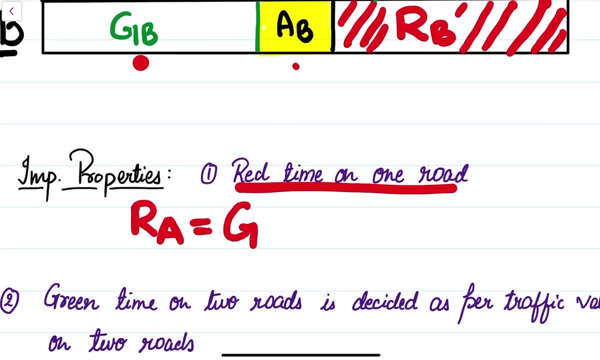 Red time is equal to the green time and amber time of the other road. So red time at road A will be the green time in road B plus amber time in road B. All right, Let us say this is our equation 1.. 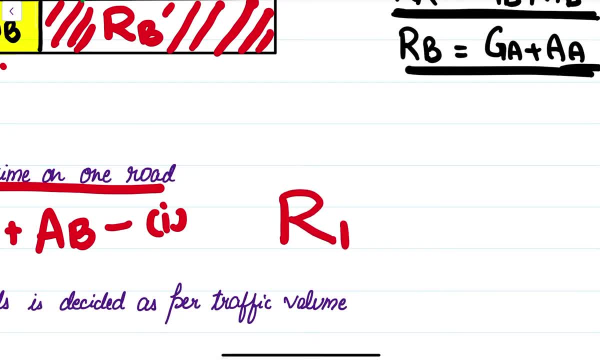 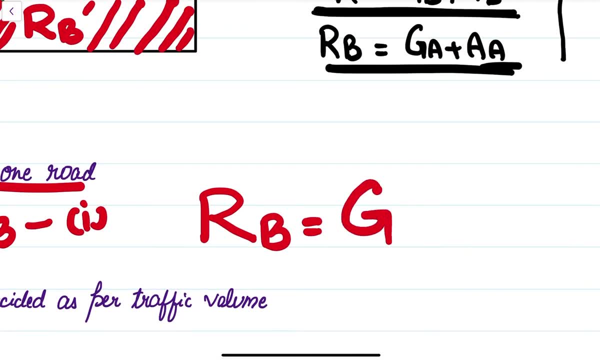 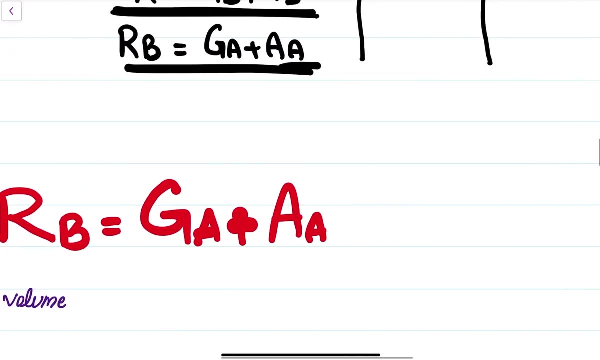 In a similar fashion, red at road B will be equals to green time in road A. Okay, In road which one? Road A plus amber time at road A. Let us say this is equation number 2.. This is equation number 2.. 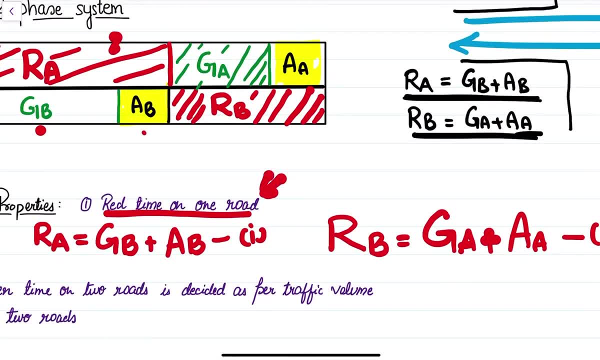 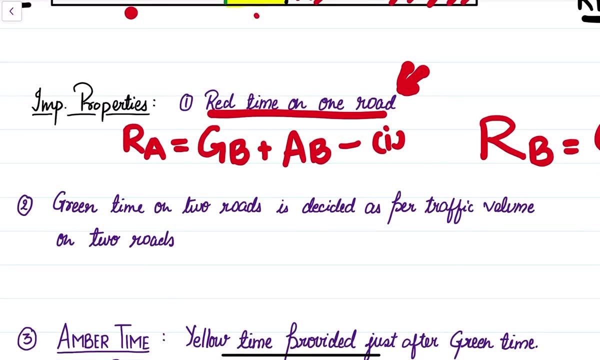 Right. So this is how the red time of one road is decided. Red time at road A will be equals to the green time and amber time of road B and likewise. Now, green time on two roads. How do we decide the green time of two roads? 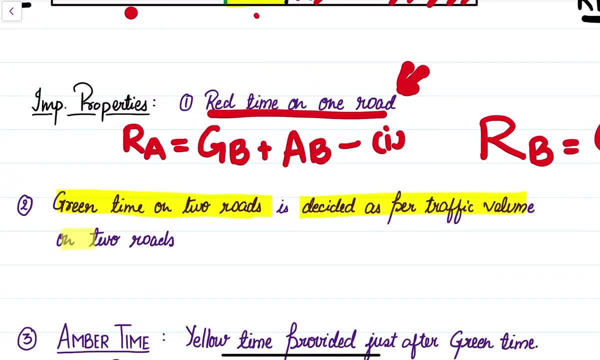 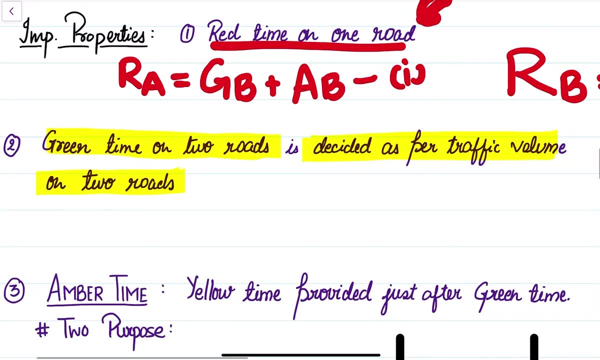 The green time of two roads is decided as per the traffic volumes of the two roads. The green time of two roads is decided as per the traffic volume of two roads. This means that green time at A is to green time at road B is equals to the traffic volume. 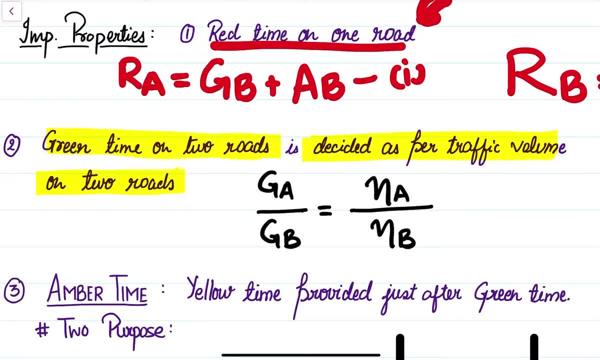 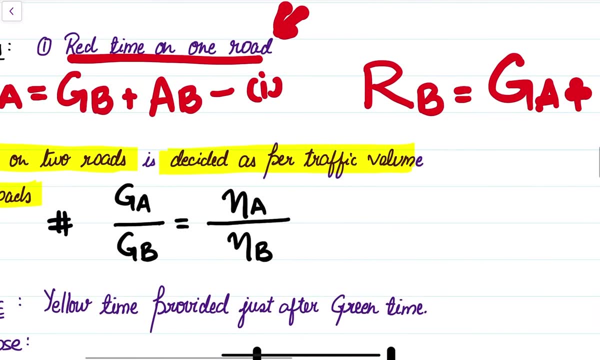 road A to the traffic volume in road B. very important relation Green time is to green time at road A to green time of road B will be equal to the traffic volume in road A to the traffic volume of road B. So I will just write down here this: N A, N, B is the traffic. 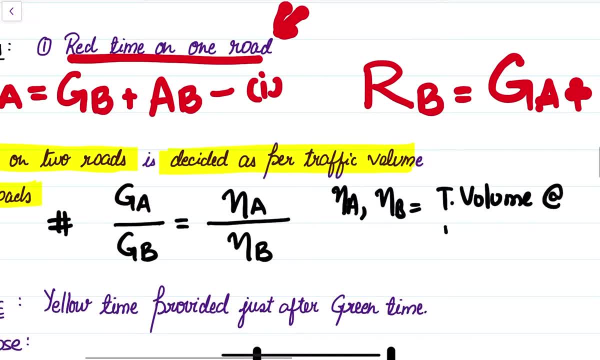 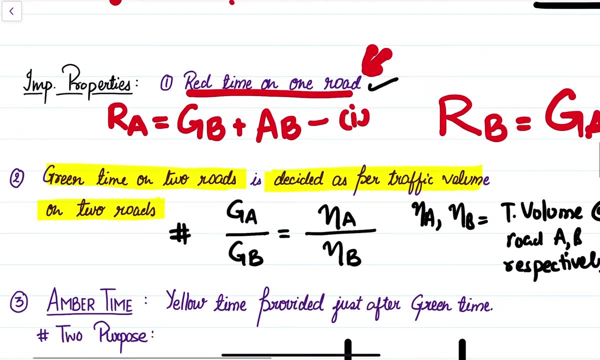 volume at road A- B respectively. The traffic volume at road A- B respectively. So we have discussed about the red time, the parameters or the relation for the red time, as well as the relation for the green time. Now let us discuss about the amber time. Let us discuss: 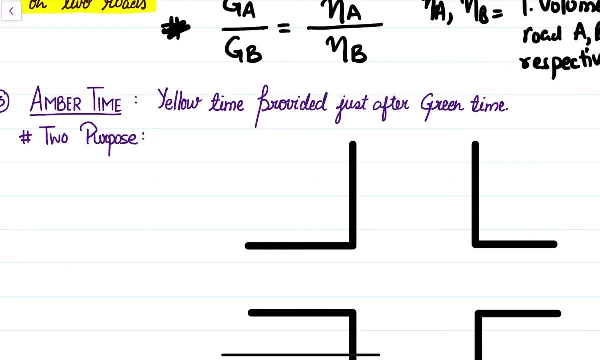 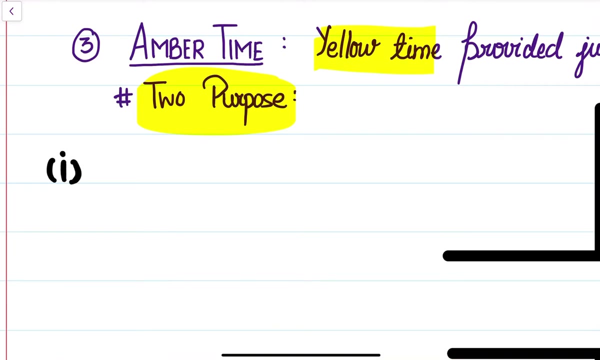 about the amber time, Yellow time, whatever you want to call it, I will refer it as the amber time, So amber time, the purpose of amber time. amber time basically serves two purposes. There are basically two purposes for amber time. The first, the first purpose. what is the first purpose of? 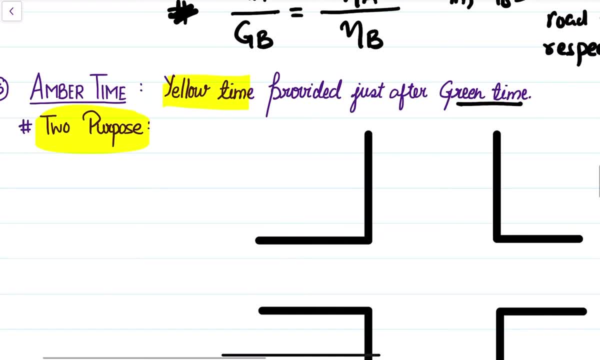 amber times. So this amber time is provided just after green time. The reason for providing it after green time, the number of times that is most meant is 5 hours. So for the number 8 hours, the 12 hours worth of green time is 32 hours. The number of hours this is 21. 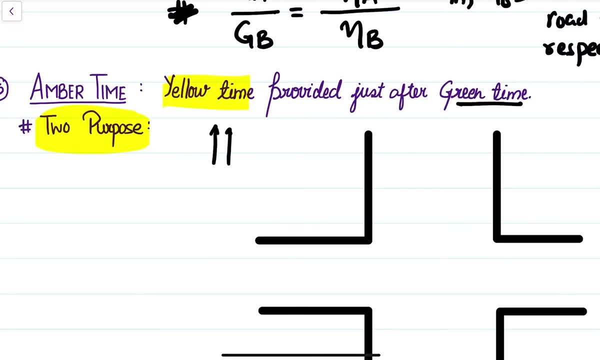 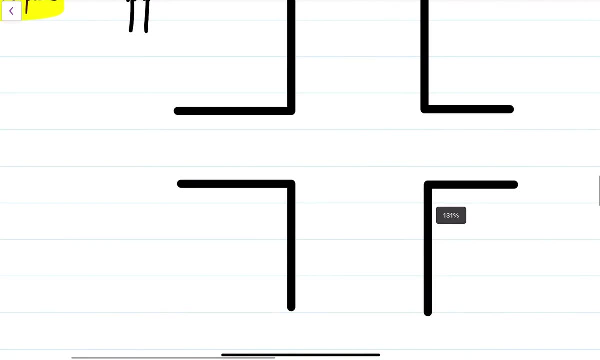 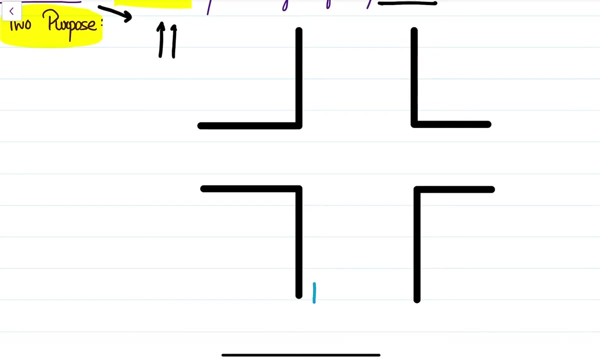 mean time is that all the vehicles that are in motion in a road when they see amber light, they get a warning right that now, in 5 to 5 to 7 seconds, there will be a red light. so we have to stop right. so in a intersection, in an intersection, in an intersection when a vehicle is moving and 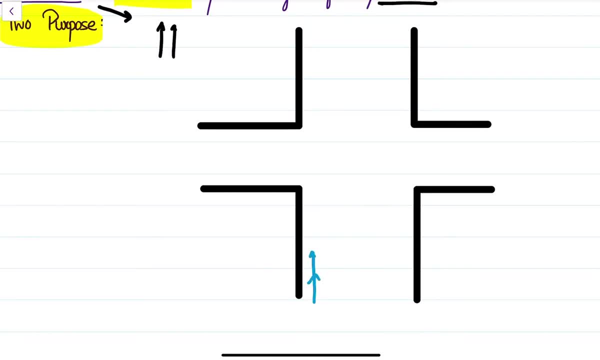 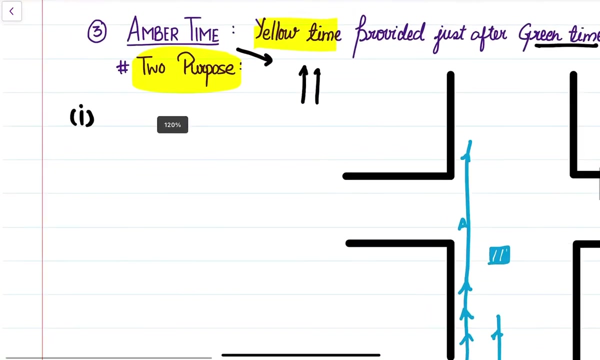 this moving vehicle. this moving vehicle sees an amber light, so it has two options. it has two options: either to speed up and cross this intersection point before the red light hits, or move as it is moving. just stop at the intersection point, right. so the purpose or the timing for the amber time should be decided in such a way that, if a 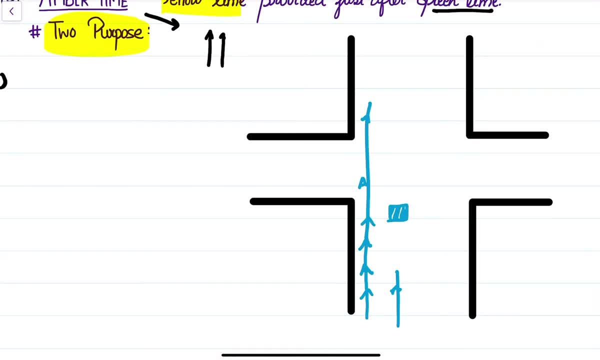 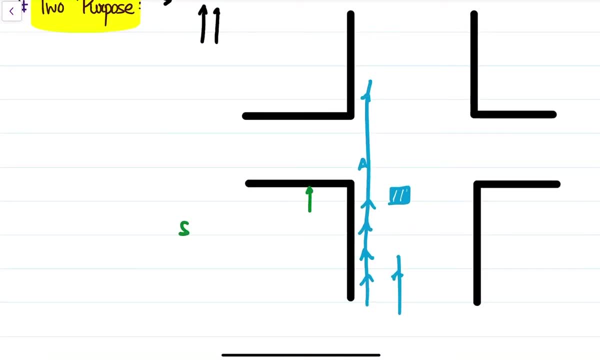 way girl wants to Bake. if it is in a zone, that is what we are going to refer it as the stopping side distance. let us say this will be, if you did stopping right distance, right. let us say this intersection distance zone is the stopping side distance. So what we want the amber time to be is if 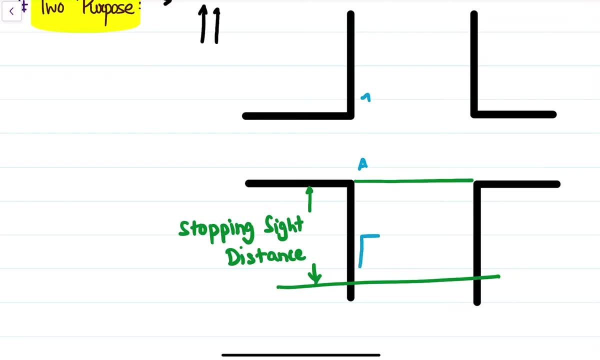 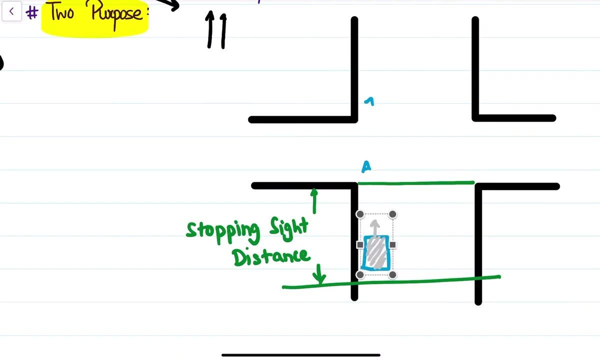 a vehicle is within this stopping side distance zone that is moving in this road. if the vehicle is within this stopping side distance, then if the vehicle sees that now it is amber and the vehicle is within this stopping side distance zone, the vehicle speeds up and crosses this. 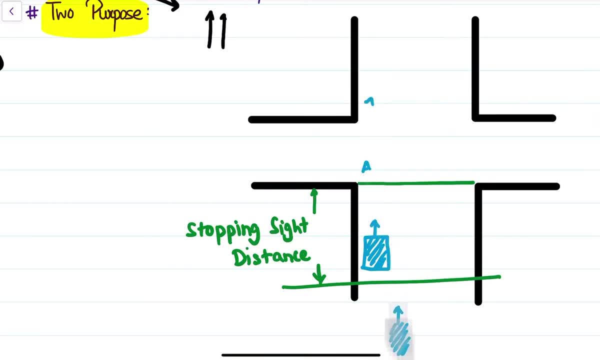 intersection point, Or if it is away or out of this stopping side distance zone, the vehicle should hit the brake and just stop at this stopping side distance at the end of the intersection. So there can be two scenarios: the amber time and the stopping time. 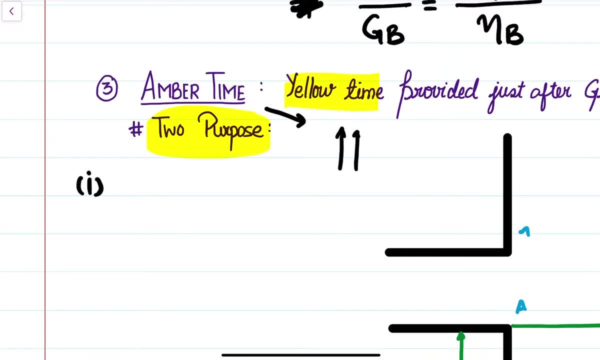 The beginning can be decided on two scenarios. The first is: the first is to allow. the first is to allow the vehicle, allow the vehicle approaching the intersection. to allow the vehicle approaching the intersection to stop between the intersection. this intellectually suggested braking to stop at this approaching side distance point is eat an amber time. to allow the vehicle reaches the points allowed at this current stopping side distance. And this appropriate braking can also be done by leading the vehicle to a portable braking SBS to allow the vehicle in advance of the taken lane lane. So it is apple time back on point. 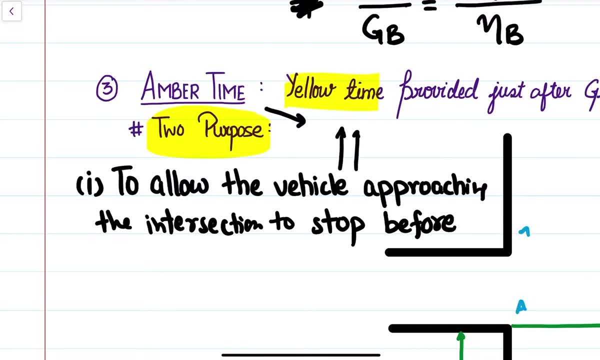 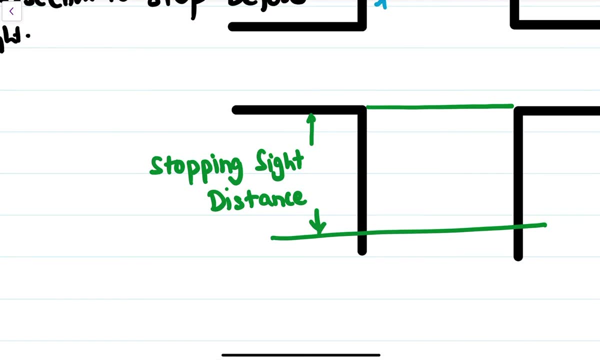 before red light, right? So what we want is that the first scenario that we are going to consider is that, right now, the vehicle is outside this stopping sight distance. the vehicle is outside this stopping sight distance and what we want is that this vehicle has. 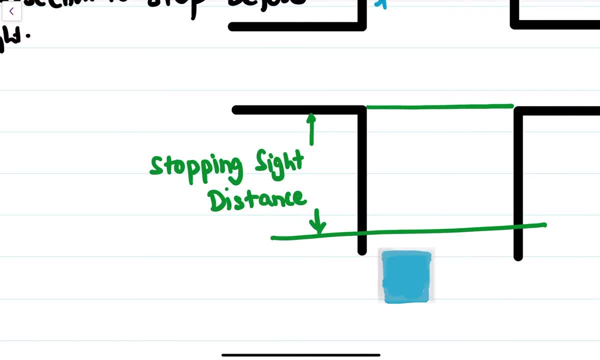 now seen that now it is going to be like the amber time: the yellow light has come up and now it will soon be red. So the vehicle that was moving. we want that as soon as the vehicle sees the amber light, it hits the brake and it stops. just at this point in between the 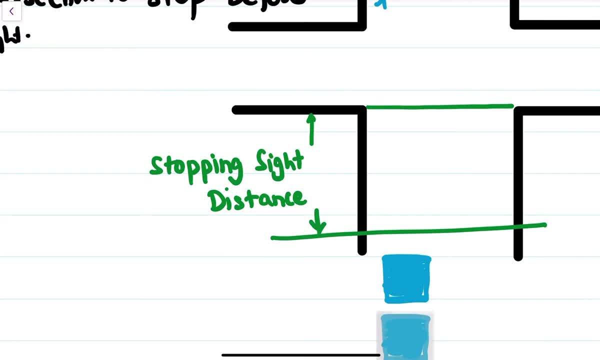 SSB zone, the stopping sight distance zone right. The vehicle is outside the SSB zone and it sees the amber light and it stops at this point right So the vehicle is outside the SSB zone. right So the vehicle is outside the SSB zone and it sees the amber light. and 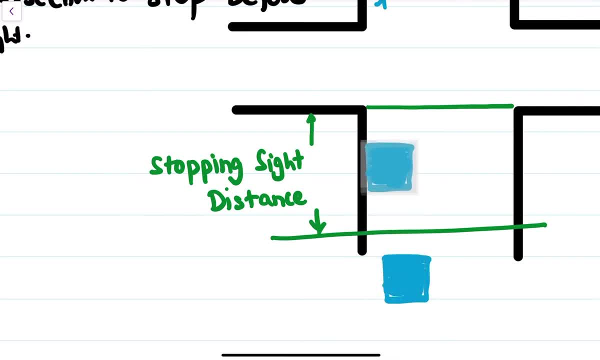 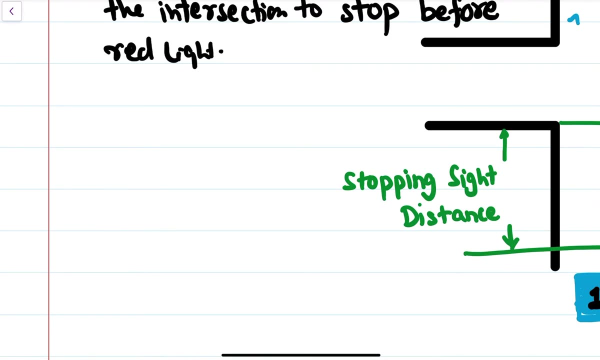 it hits the brake and it should just stop here, right, at a safe distance. Right, this is what we want. Right now, the vehicle is outside the SSB zone. This is the case number 1.. So, to do that, to do that, let us say, let us say the design speed of the vehicle. 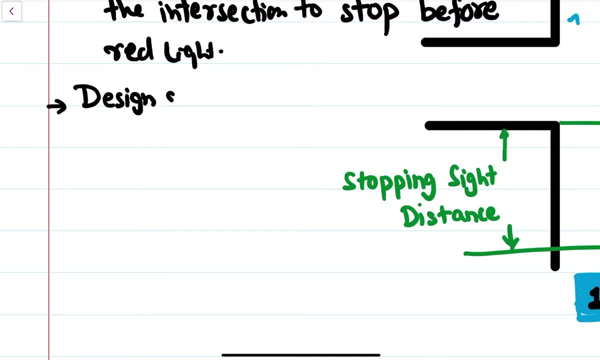 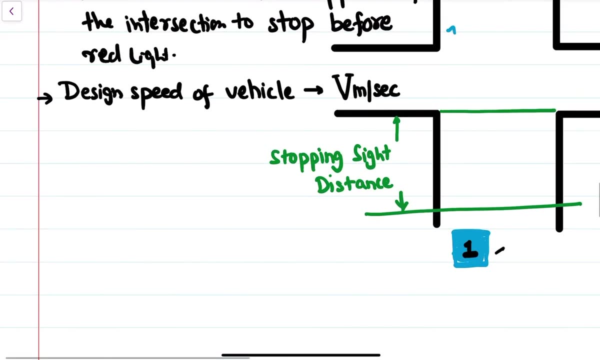 is V. The design speed, design speed of the vehicle is V. So the design speed of the vehicle of the vehicle is a Vmeter per second. The design speed with which this vehicle is moving is Vmeter per second. So now the vehicle starts to hit the brake right, So it will. 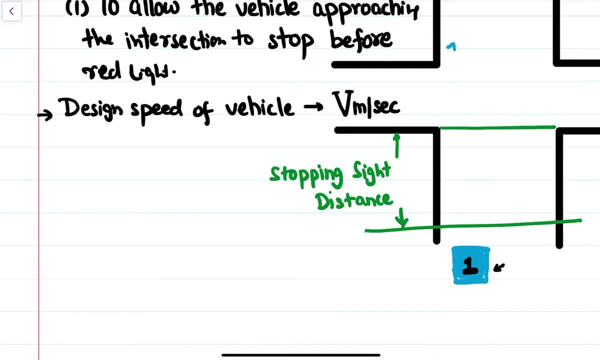 decelerate, it will retard with certain with or with certain negative acceleration. right So the retardation. let us assume the off heavy curve. so for a sidey centre, or for a sidey centre, right, Okay. So what will happen? What will happen? Okay, If ifädiding to the centre of a cart, 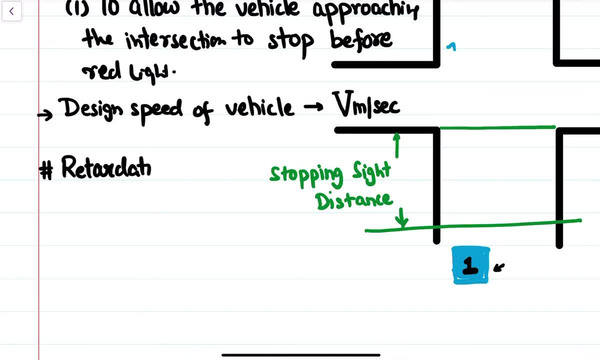 retardation to be minus A. right, The retardation is minus A, So it was moving with certain velocity, it was coming or approaching the intersection with certain velocity and it sees the embolite, it hits the brake and de-accelerate, de-accelerate, de-accelerate and stop right. 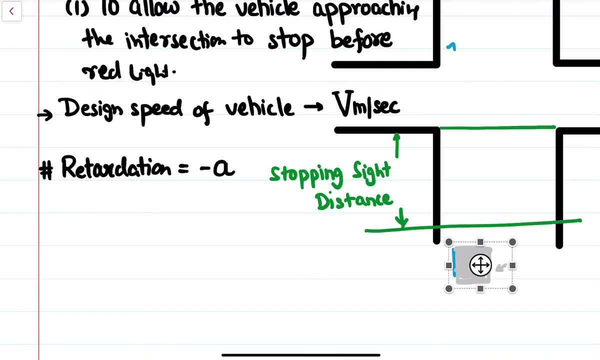 So this the final velocity of this vehicle is 0, right, So we already know v equal to u plus at in this case, since it is de-acceleration, so it is minus A. So minus A the final velocity. 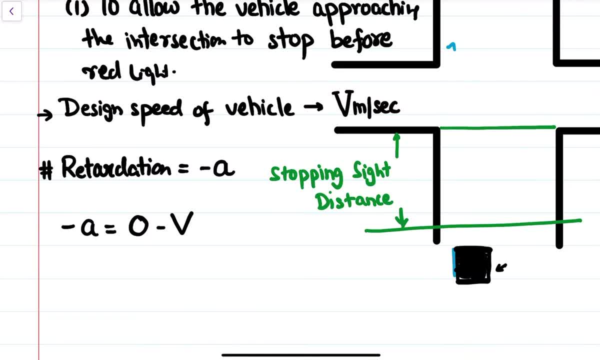 is 0, the velocity with which it was moving is the design speed. that is v, and it takes time, t. So the value of t will be v by A. t means the ember time, the ember time that we want to be, that safe time at which the vehicle can safely de-accelerate and stop here right. 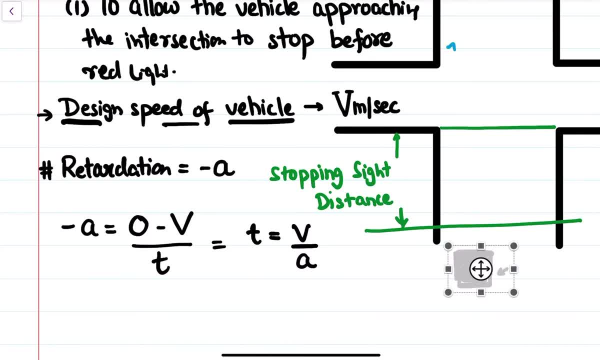 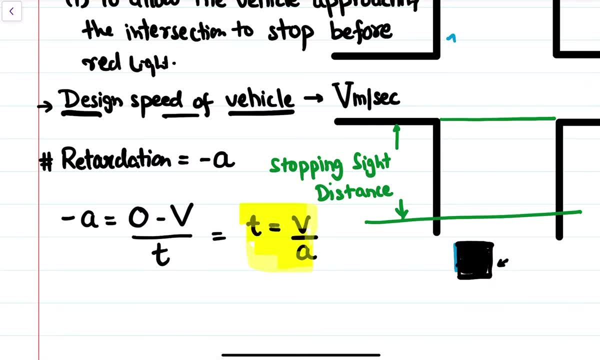 That is the time period of the ember time that we want, right? So that is, this is the one factor that is We are going to consider Now. this ember time will also include one parameter called as the reaction time, tr. that is called as the reaction time because, because the vehicle 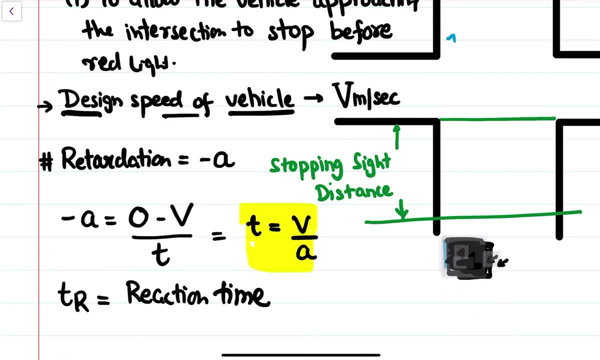 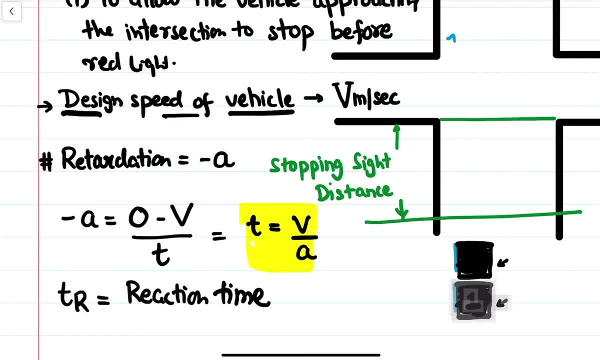 the light turning ember, it anticipates, it reacts to this situation and then it hits the brake Right. It takes certain time, tr- to react to this right, And then it hits the brake, It de-accelerates, reaches to the final velocity to be 0, and stops here. 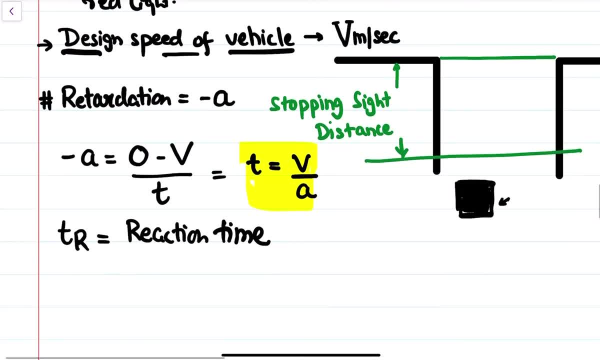 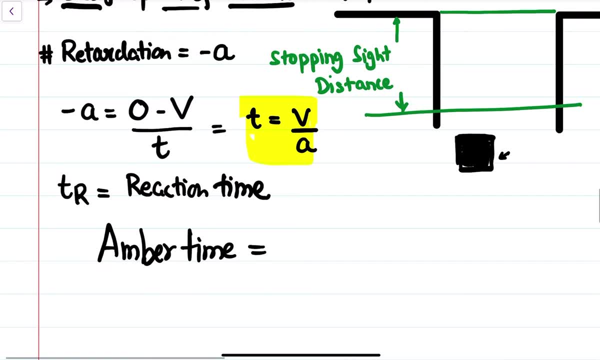 Correct. So the overall ember time, the overall ember time, if we want to say the overall Ember time in this case, in case where the vehicle is outside the SSD zone, the stopping side distance zone will be T R plus T, T R plus T, that is the reaction time to react. 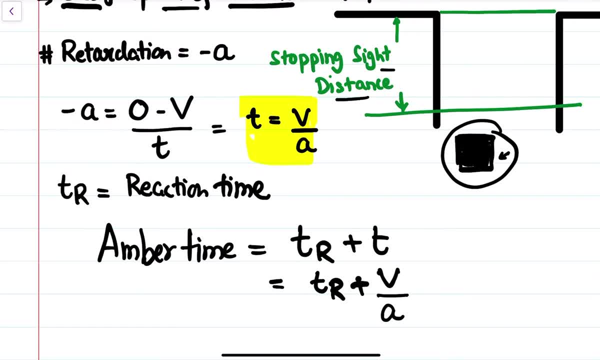 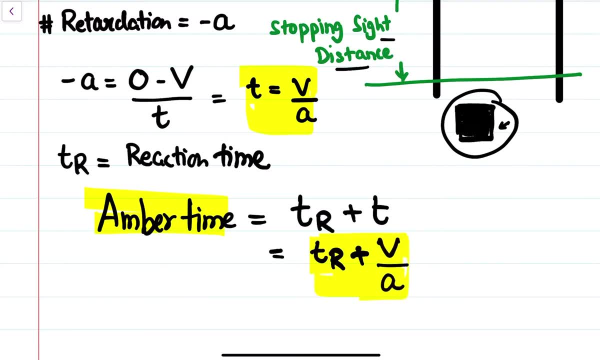 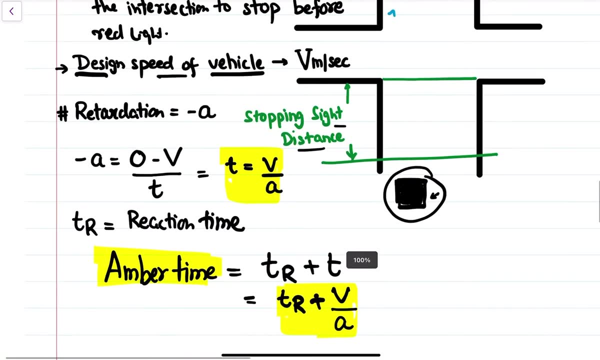 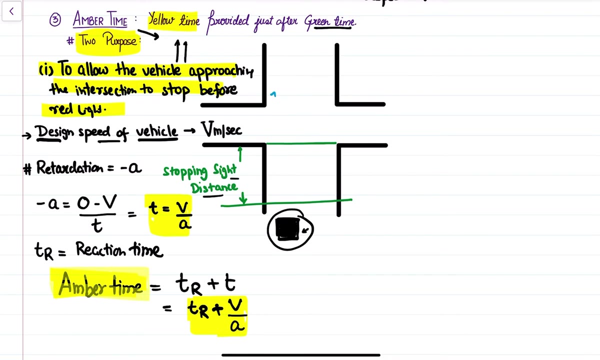 to this situation, plus V by A. So this is the one situation that is by which the Ember time is decided. Ember time for case 1 will be T R plus V by A. I hope it is clear. So the first purpose has been achieved. The first criteria of the Ember time is T R plus V by 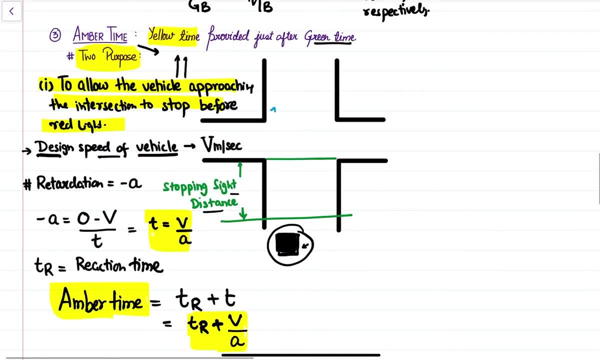 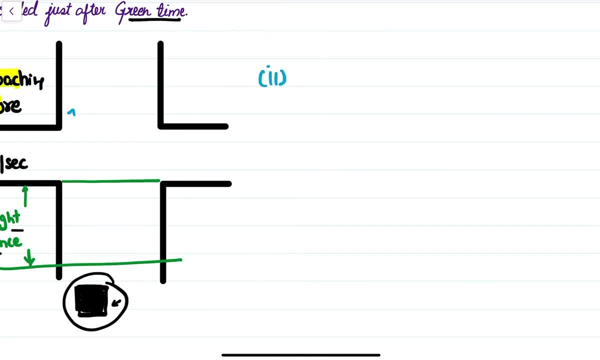 A. Now let us discuss about the second criteria. Now let us discuss about the criteria number 2.. Now in criteria number 2.. Now let us discuss about the criteria number 2.. Now in criteria number 2.. Now in criteria. 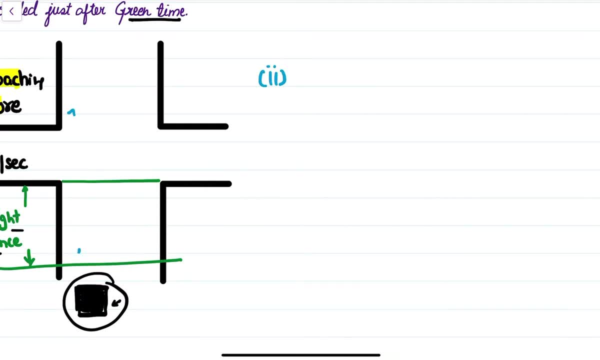 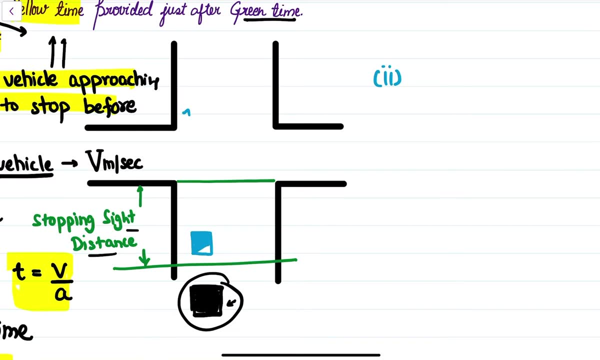 what we have is we have the vehicle within the stopping side distance zone, right, we have the vehicle within the stopping side distance zone and, of course, the vehicle is in motion right now. the vehicle is in motion right, it is moving within, in this stopping side distance zone and we want that, all the vehicles who are in this SSD zone, we want as soon as the. 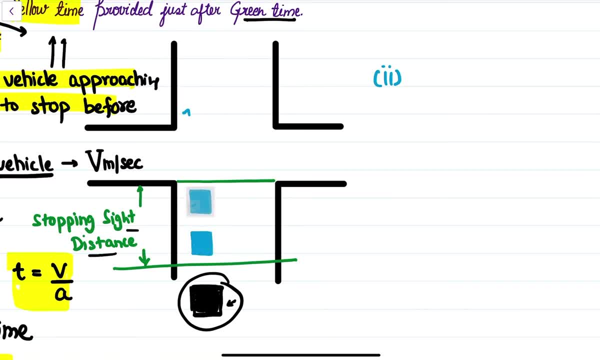 vehicle sees the amber light, they speed up and they cross this intersection safely right. we want to set the amber time in such a way. the case number two should be that amber time should be in such a way that the vehicle that are within the SSD zone, within the stop starting side distance. 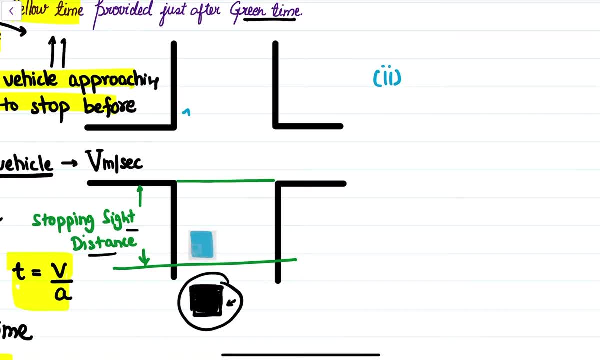 zone. if they are in this zone, they should accelerate and should cross this intersection safely and be shared before the red light hits. so what are the parameters that we should consider? so let us say: the width of this road is w. right, this is the. this is the width of the road w. so what we want is: 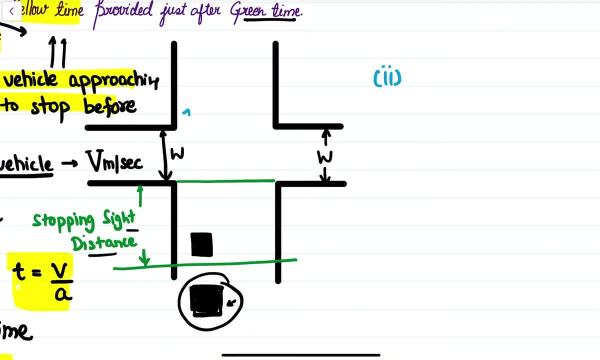 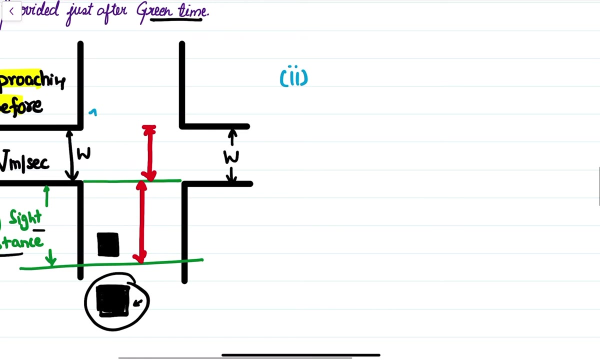 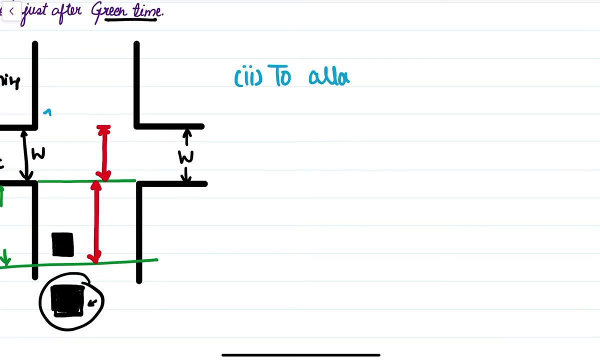 we want that the vehicle should cover this distance as well as this distance, correct, we want the vehicle to consider this, to cover this distance. so the amber time should be sufficient enough to cover this distance, right. so the second situation should be the second criteria to decide the amber time is to allow, to allow the vehicle, to allow the vehicles. 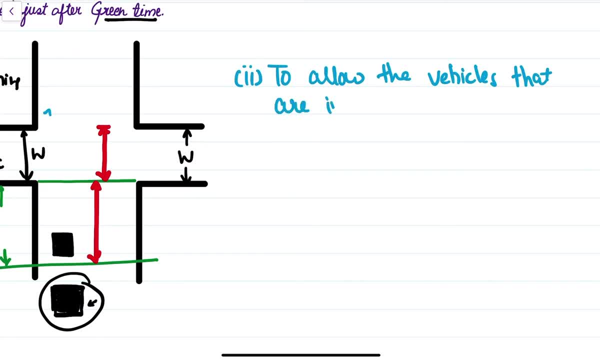 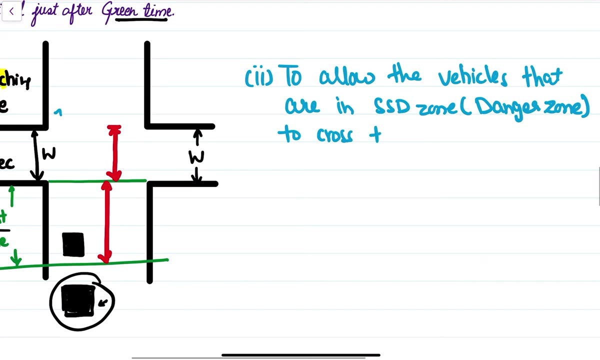 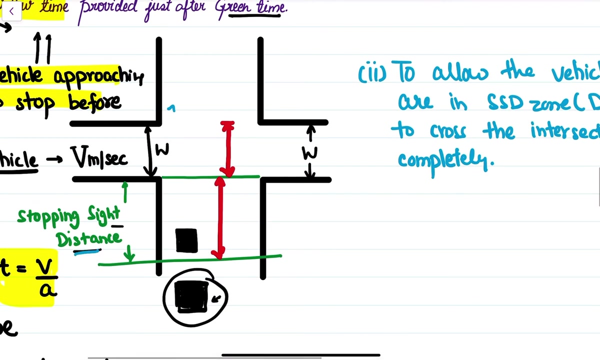 that are that are in SSD zone, that we, in this case, we can call it as danger zone, which are in danger zone, to cross the intersection, to cross the intersection, to cross the intersection completely to allow the vehicle that are in this SSD zone, which we can also call it as danger zone, in this. 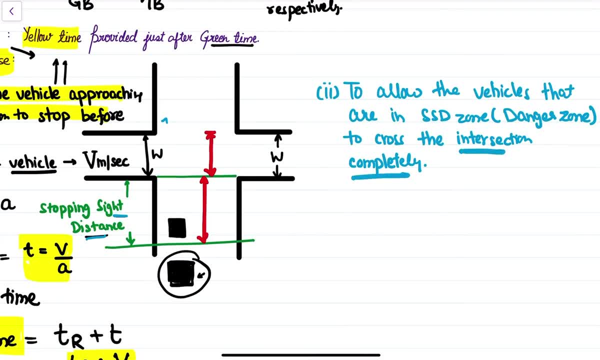 case, to cross this intersection, completely, right. So what we are interested is in the time period. time is equal to distance upon speed, right? So this is our design speed, that we have already assumed right, this is our design speed. 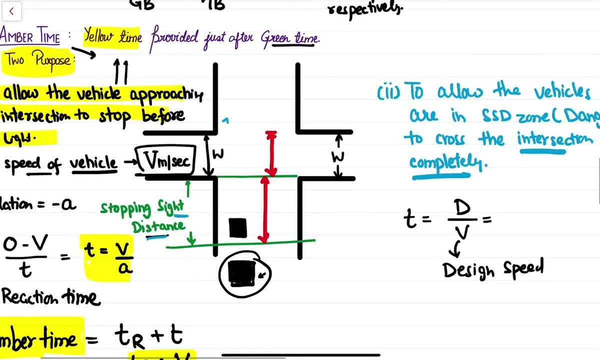 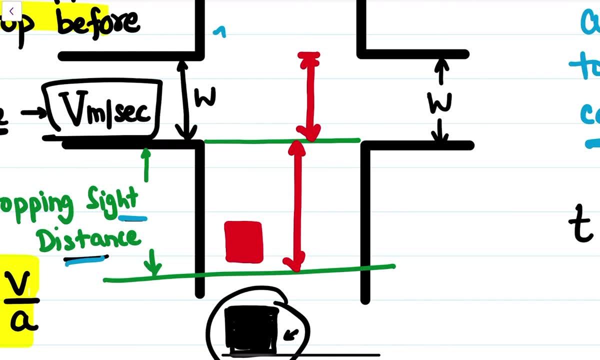 Now, what is the distance that we have assumed, Right? What is the distance that that is needed to be covered, right? What is the? what is the distance of this vehicle that is in danger zone to be covered? The first is this SSD zone and second is this W, correct? 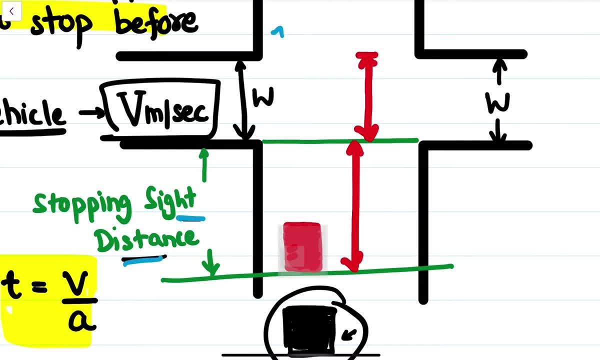 But if you observe, so let us say vehicle is in this SSD zone, so the distance that is covered by the vehicle is this much. then we are saying W, W is this much. But if you see, here the vehicle is still at this point, right at red light, the vehicle. 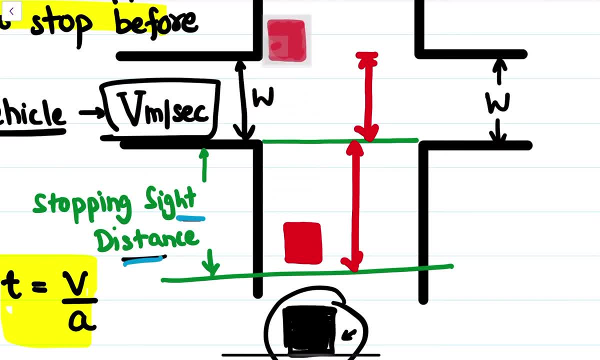 is here. It has not completely crossed Why? The reason is we have not considered the length of the vehicle. that is why, right, we have not considered the length of the vehicle. I will again repeat: If the vehicle is in this SSD zone, the vehicle is in this SSD zone. this is our SSD zone. 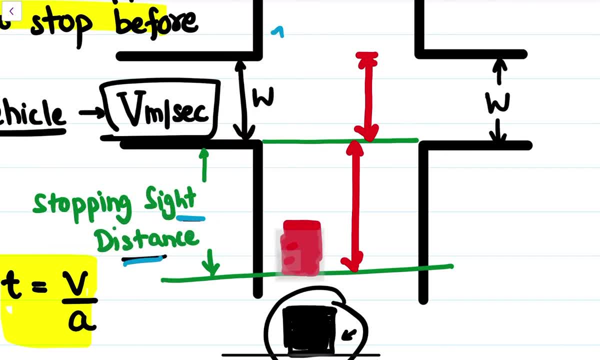 this is the wheel, right, So this is the wheel. So this is the wheel. Now the vehicle has to cover this whole section so as to be safe. right, the vehicle has to be here before the red light hits, because as soon as it is red for this road, the vehicle 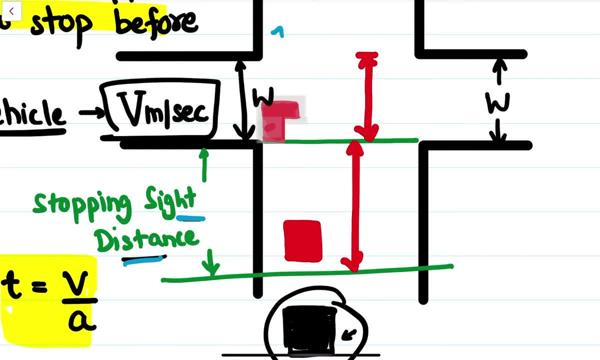 from this road will start to move right. So we want the vehicle to be here, our vehicle to be here. So the distance that it has to cover, SSD, then W right. but if you see the end or the 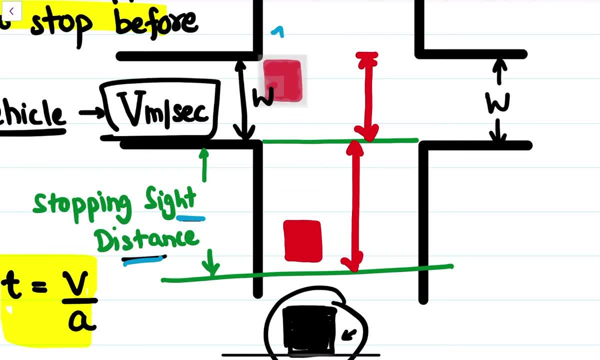 rear of the vehicle is still in between the concrete zone. So if we consider the length of the vehicle, L, then the vehicle is has covered the required distance, correct? So if we say, let us say if L is the length of the vehicle, if L is the length of the 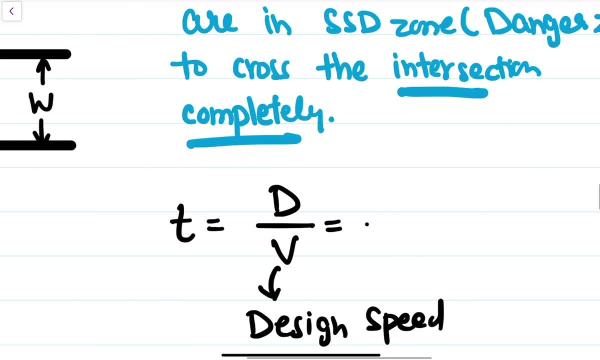 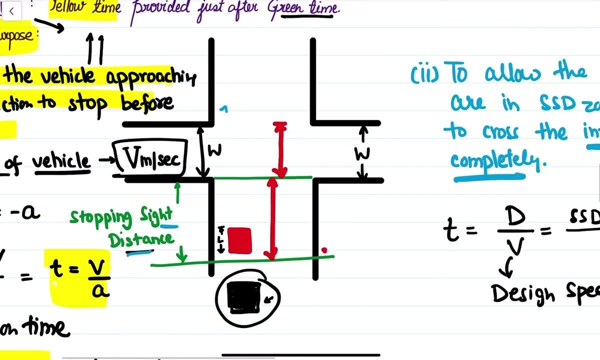 vehicle, Then the total length of the vehicle is L, Right, Right. So total distance the vehicle has to cover is the SSD plus the width of the road- W, and the length of the vehicle: L. clear The vehicle has to cover the, this SSD, this path, this width of the vehicle plus the length. 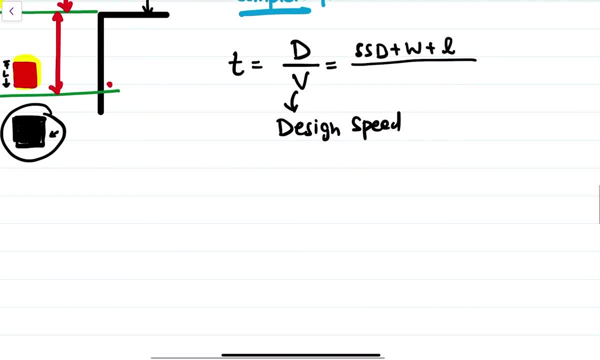 of the vehicle, So T will be equal to. T will be equal to SSD plus the length of the vehicle, So T will be equal to T plus W plus L by V, right where L is the, L is the length of. 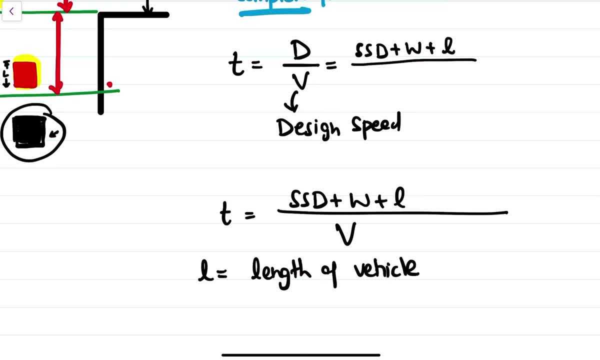 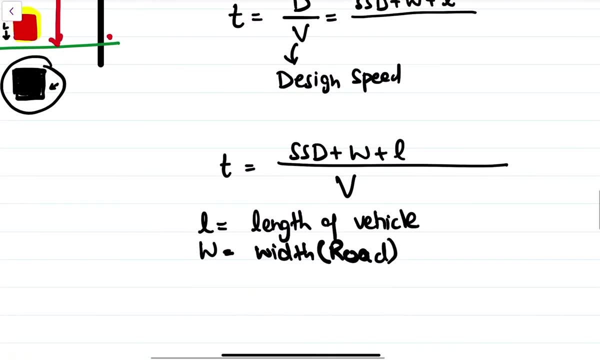 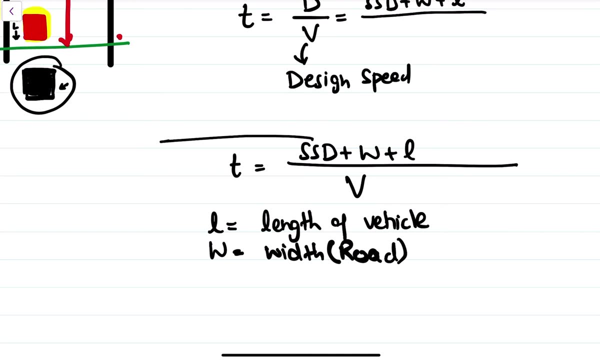 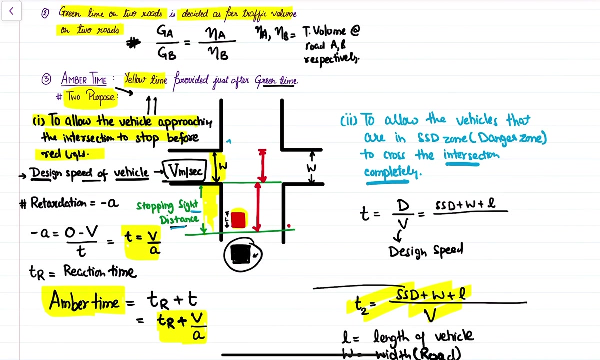 vehicle, W width of road and SSD is the safe stopping distance. right, So this is our T2,. right, This is our T2.. So, this is our T2.. Right, So this is our T2.. So these are the two criteria, that on which the amber time, this amber time, is decided. 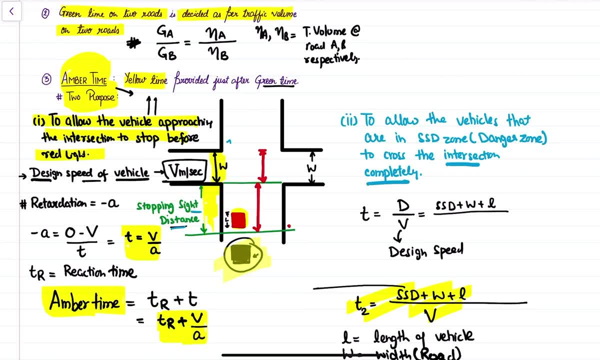 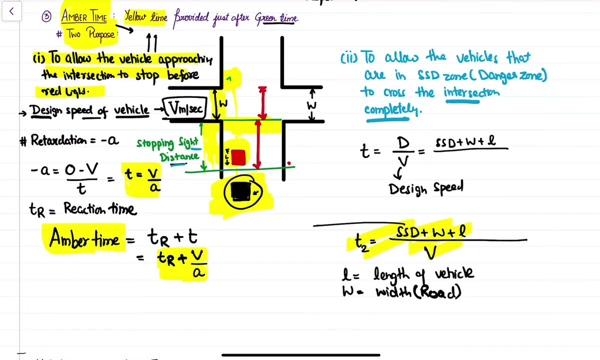 The two purposes: the vehicle that are outside the danger zone or SSD zone, it should stop right at this intersection point, and the vehicle that are in danger zone should cross the intersection point Right. So these so we have two times: one is T1, this means that it has T1 here, and second, 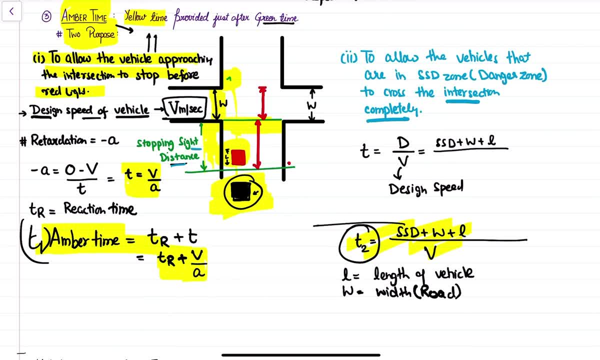 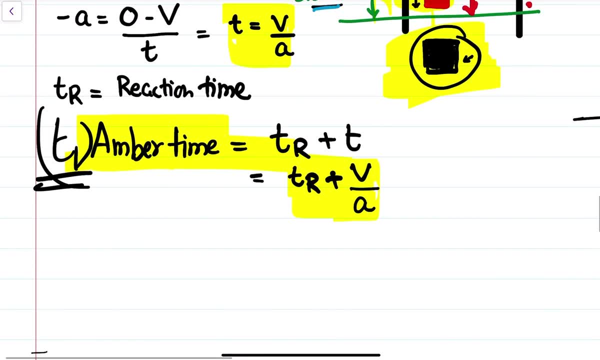 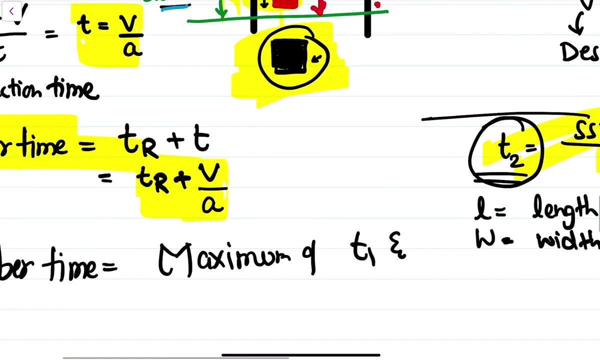 is T2.. Right, So the amber time will be maximum of these two. right So the amber time, the final amber time that we have to adopt, is maximum of T1 and T1,. maximum of T1 or T2, whichever is the maximum that we have to take. 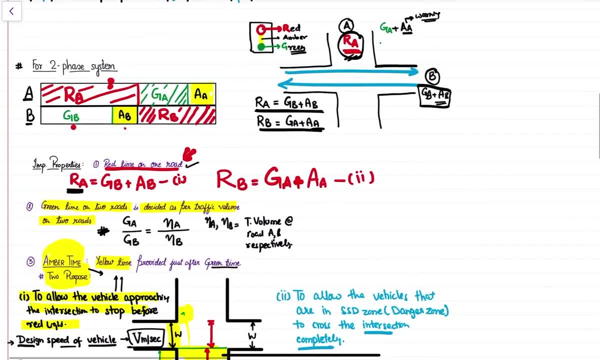 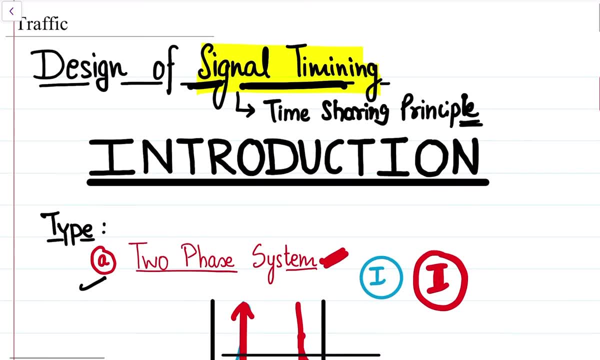 Right, So these are the two basic criteria that are taken into account for the design of signal timing. These are the basic criteria that are taken into account for the design of signal timing. Alright, So I hope these basic criteria are clear to you, right. 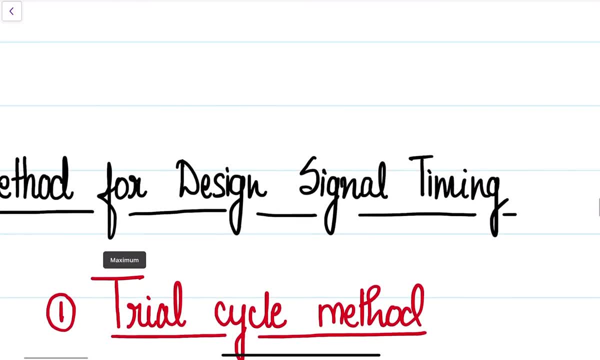 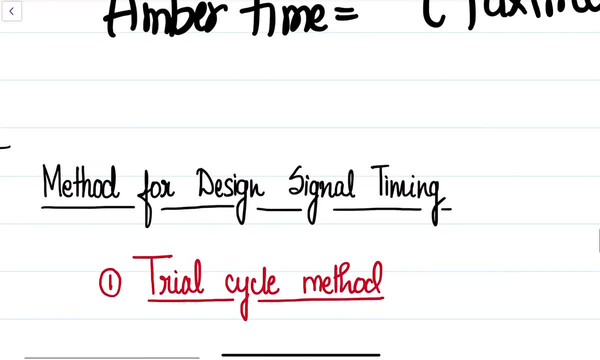 In the upcoming lectures we are going to discuss about the methods for the design of signal timing. Basically we are we are going to discuss like four methods. One is the prior cycle method. second is the approximation. third is the Webster's method. 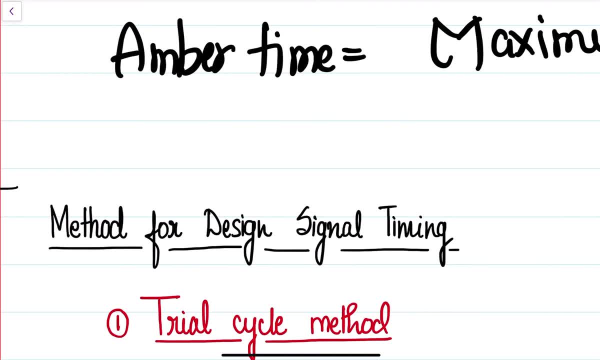 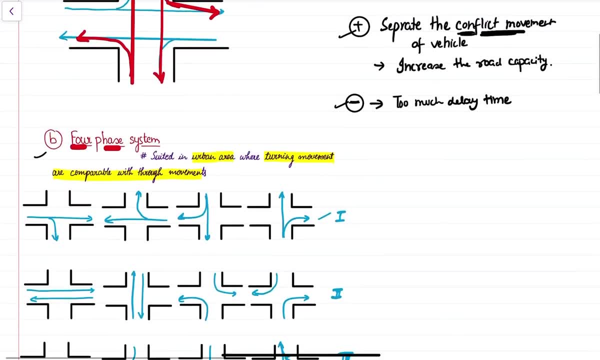 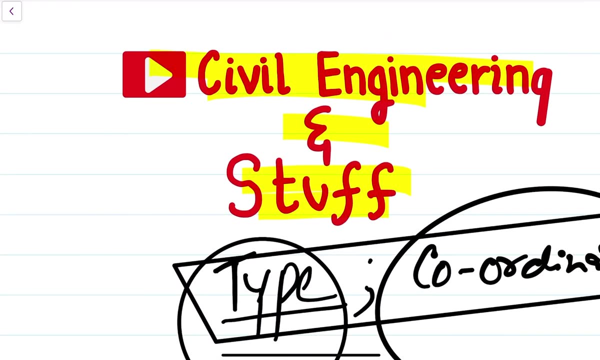 and fourth is the IRC method- Right method- which is a combination of approximation and vector, so we are going to discuss at that point of time. okay, so this is the basic about the design of traffic signal timing, right? I hope the lecture was useful to you, right? and, like I always say, if you find this video,